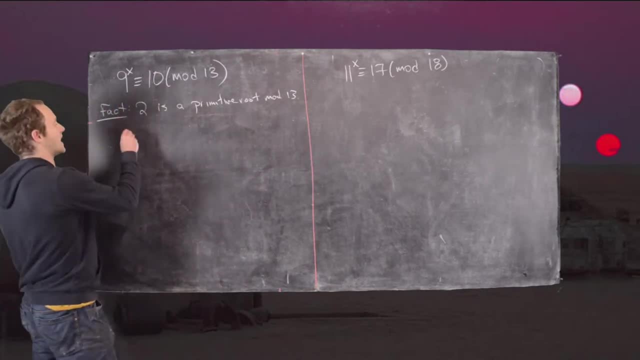 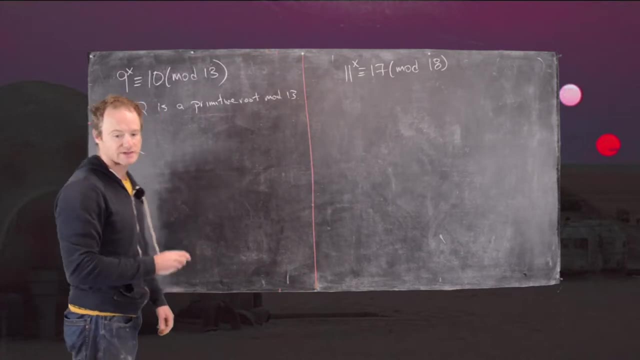 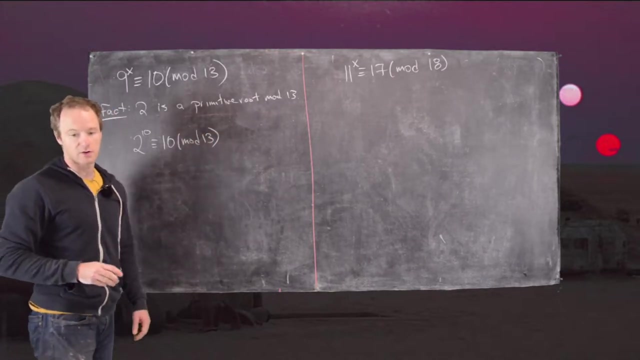 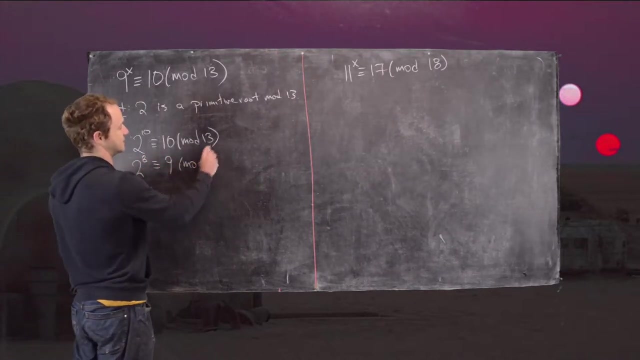 So I'll skip the details. But you can show that 2 to the power 10 is congruent to 10 mod 13.. And also 2 to the power 8 is congruent to 9 mod 13.. And so you can do that just by checking all the powers of 2 until you get up to these appropriate numbers. 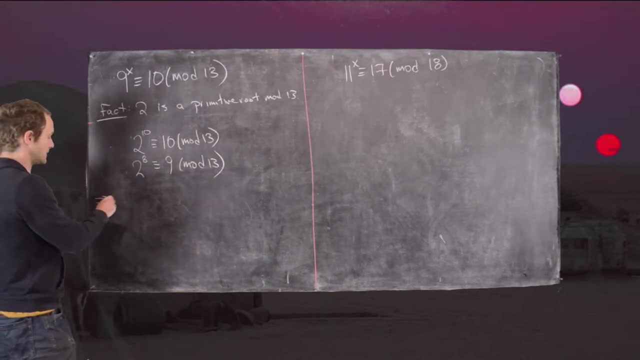 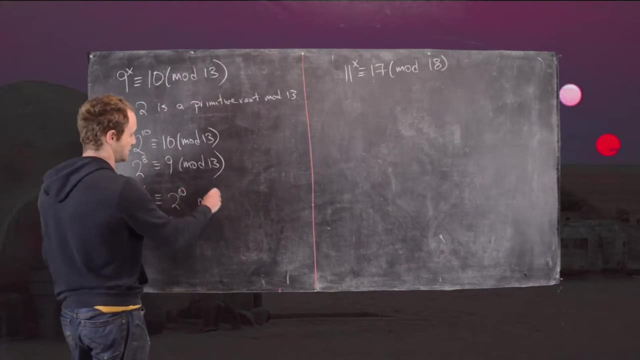 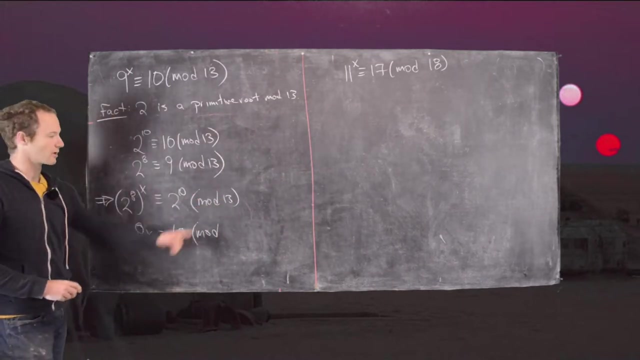 Okay, good, So that's going to turn this equation into the following: So we have 2 to the 8 to the x is congruent to 2 to the 10 mod 13.. But that tells us 8x is congruent to 10 mod, but now, since we're working in the exponent, we're not mod 13 anymore. 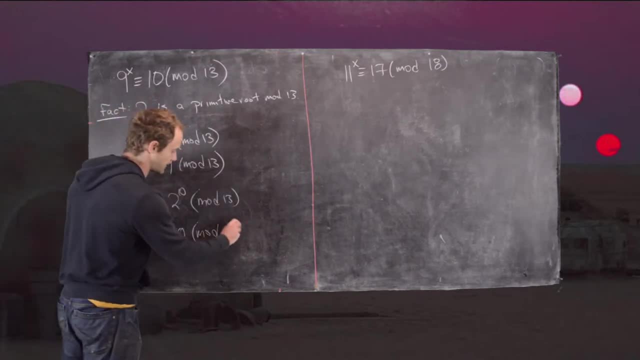 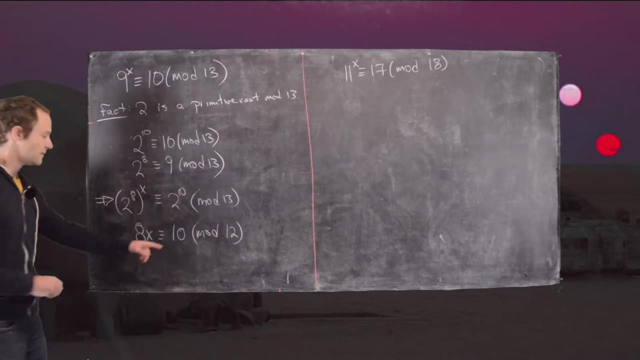 We're mod the Euler phi function of 13,, which is 12.. Okay, good, So now we have 8x is congruent to 10 mod 12.. But notice, this has no solution, and that's because the GCD of 8 and 12 equals 4,, which does not divide 10.. 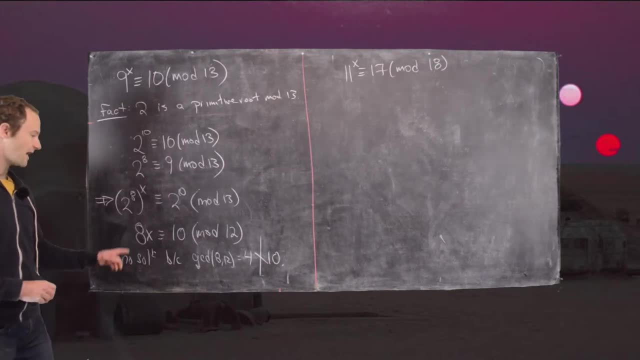 So, if you recall, in a previous video we proved that if the GCD of this number, this number, divides this number, that's precise. That's a precise way of deciding whether or not this has a solution or not. So in this case, we don't have a solution. 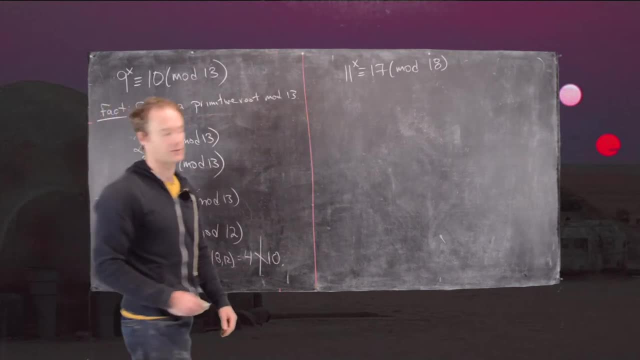 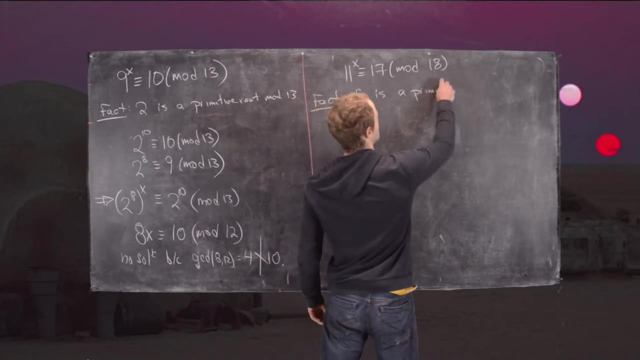 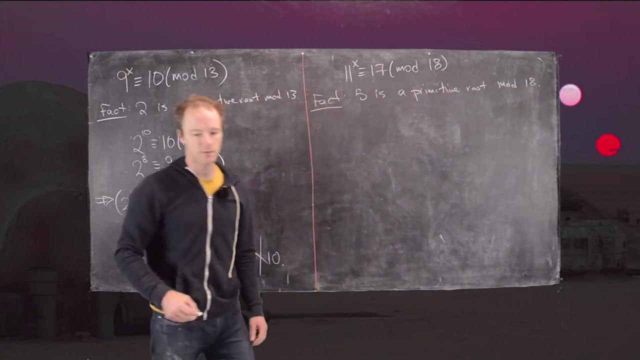 Okay, good, So now we're going to move on to the next one. So again, we know there's a primitive root, and I'll just say fact 5 is a primitive root, Mod 18.. And we can also notice the following, and that is: 11 is the same thing as 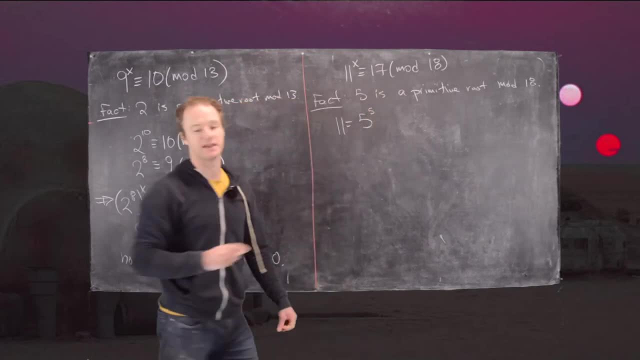 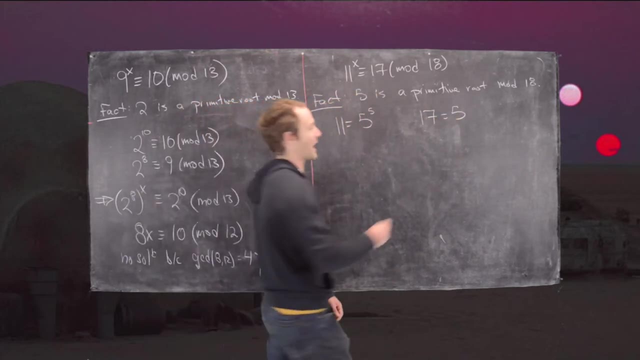 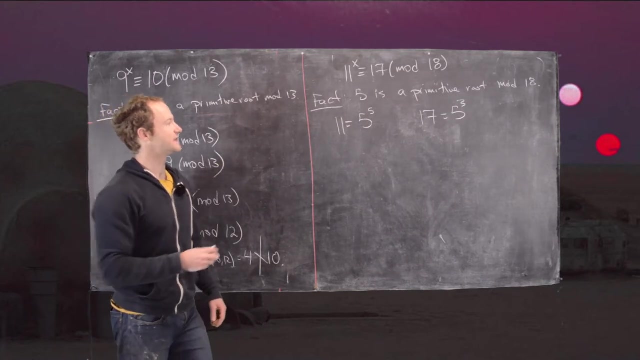 5 to the 5th power, mod 18, and 17 is the same thing as 5 to the 3rd power, mod 18.. So all those are happening, mod 18.. Okay, good, So now what we can do is the following.